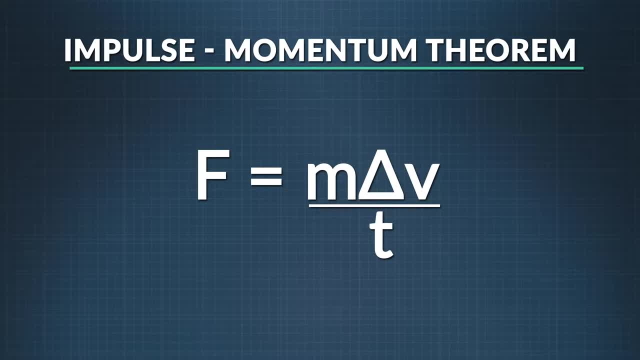 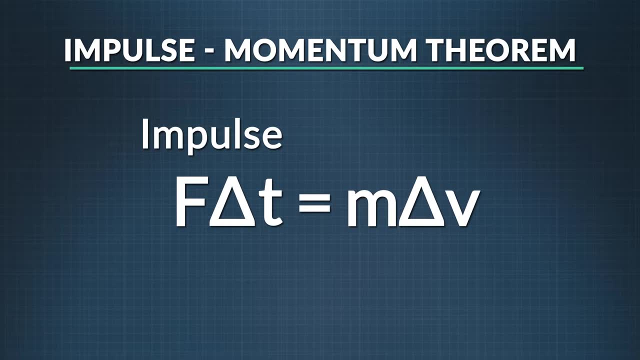 In order for an object's momentum to change, a force must be applied for a period of time. This is known as an object's impulse. The theorem says that the impulse applied to an object is equal to the change in momentum of an object. The impulse can be a larger. 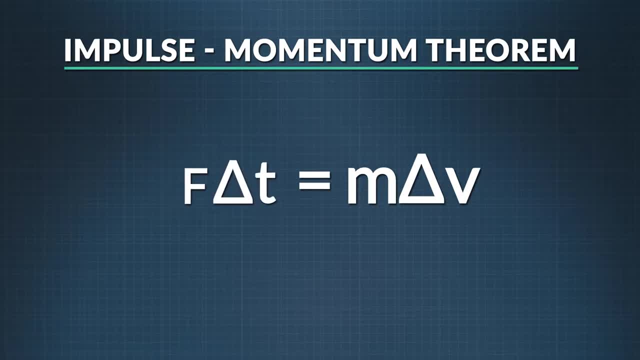 force over a short period of time, or a smaller force over a longer period of time, or some smaller force over a longer period of time. You can start to see where we're going with this When I throw the egg against the wall. what can we say about the impulse involved? It's a large force over a short period of. 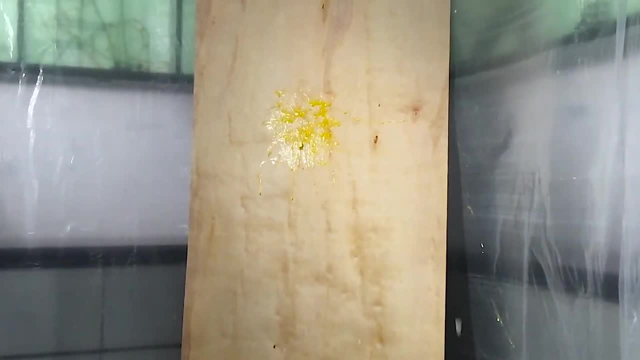 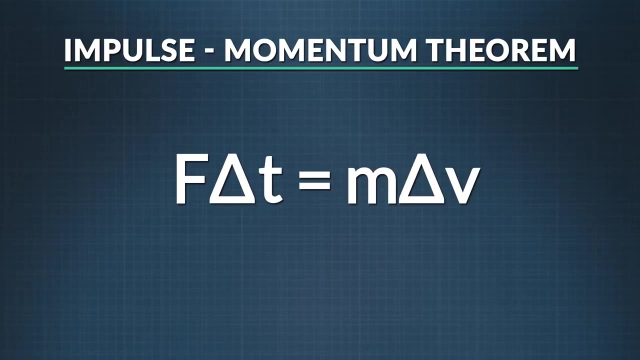 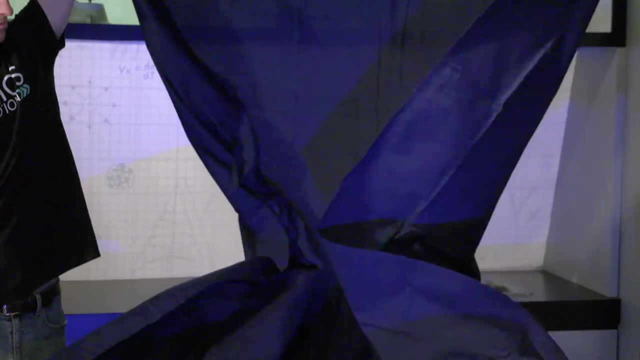 time because it hit the wall and its momentum was stopped abruptly. When I throw the egg against a sheet, do you think the force is small or large? It's a weaker force applied over a longer period of time because the sheet gives even though the impulse is the same as the force. applied over a longer period of time because the sheet gives even though the impulse is the same. 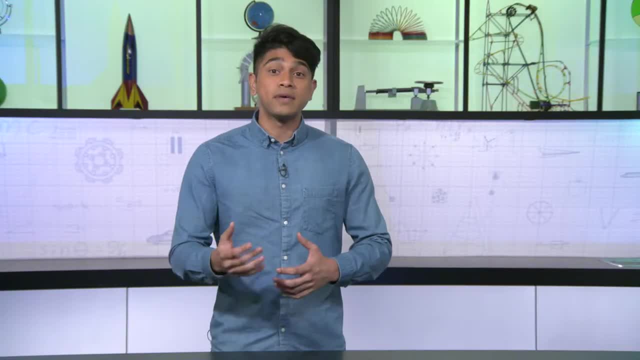 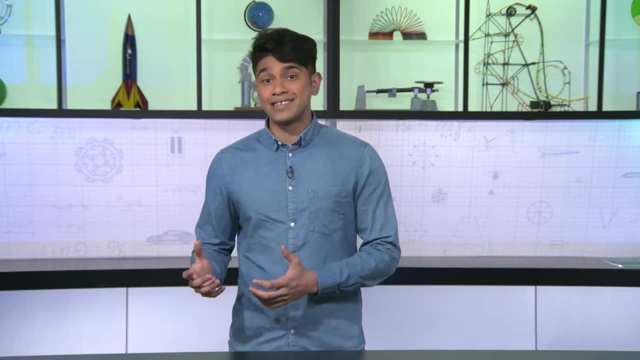 as when we throw it against the wall. the egg will not break because it experiences a smaller force. And that's the difference between throwing an egg against a wall and against a sheet. The egg experiences the same impulse in both cases, but the stopping time. 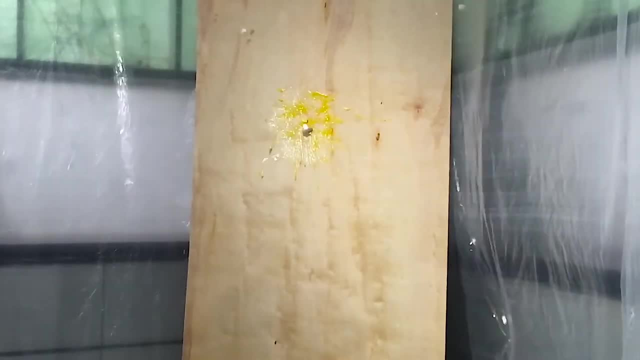 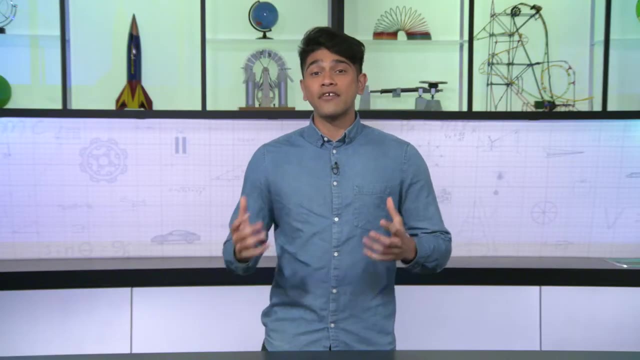 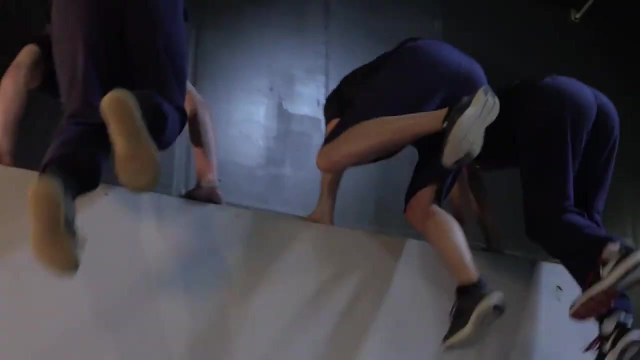 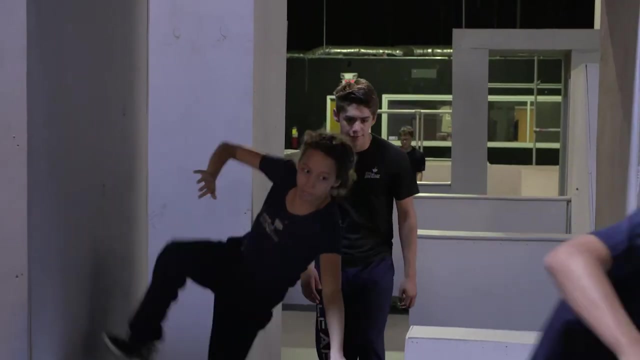 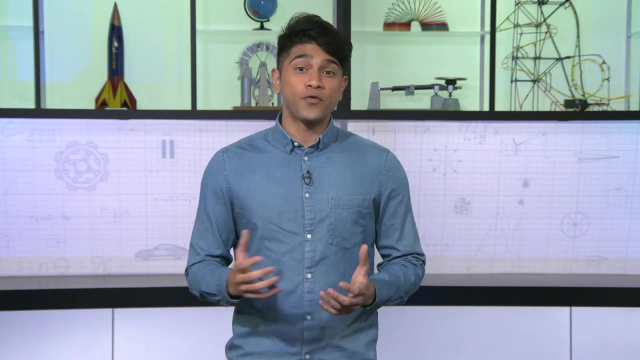 when it hits the sheet is much larger than when it hits the wall. By increasing the stopping time, the force required to stop the egg is decreased. Let's look at how athletes use momentum and impulse through an activity called momentum. Parkour or freerunning was originally used for firefighter military training, Now people. 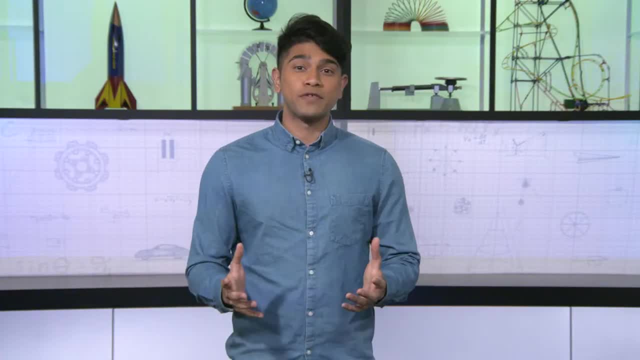 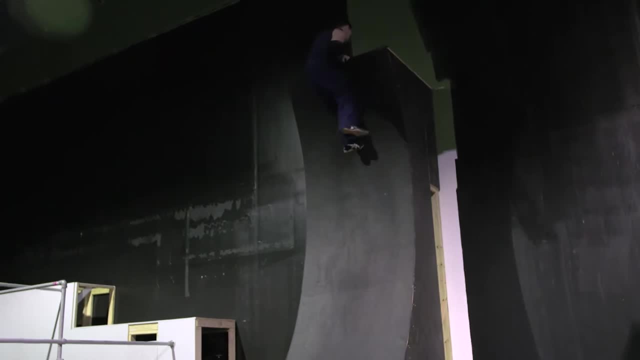 do it for fun and fitness. One of the most popular maneuvers in parkour is the vertical wall run. This is where a runner tries to reach a vertical height that a regular jump off the ground couldn't manage. He has to redirect his horizontal momentum into vertical momentum to carry him. 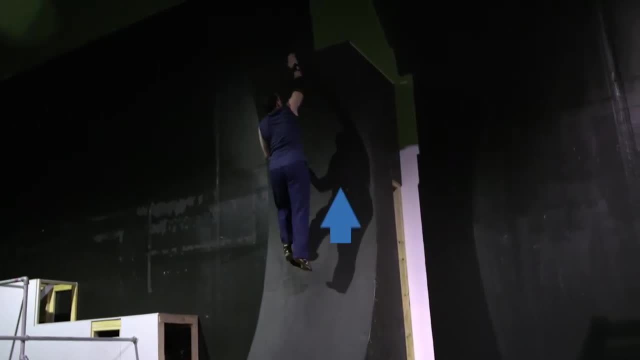 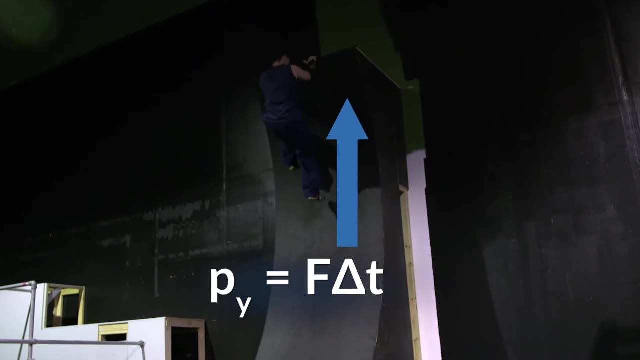 up the wall as far as he can go, and he has to max out the force he exerts over a shorter period of time as his foot hits the wall so he can climb as high as he can. No way he could have done that without momentum and impulse, And remember, momentum is a vector.